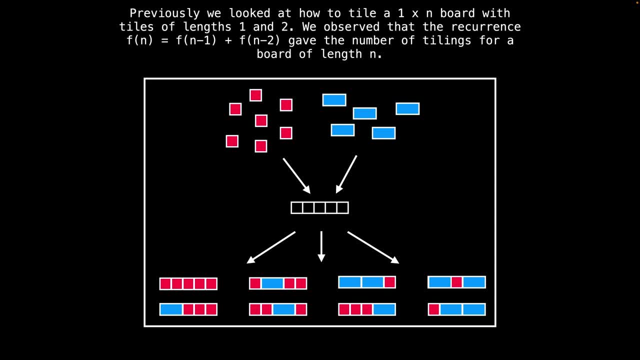 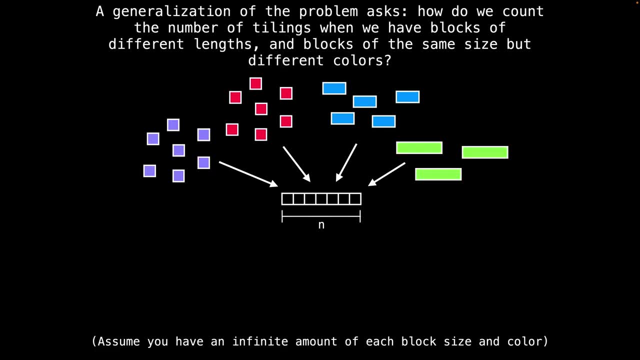 that the recurrence f of n equals f of n minus one plus f of n minus two gave the number of tilings for a board of length n. Today we're going to ask the generalization of the problem, which is: how do we count the number of tilings when we have blocks of different? 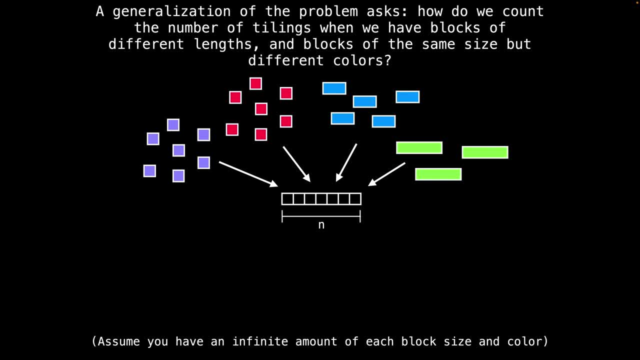 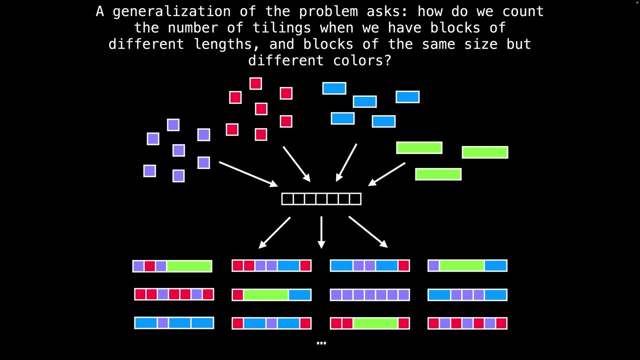 lengths And blocks of the same length but different colors. Again, you can assume that there is an infinite amount of each block size and color. For instance, as you can imagine, there are numerous ways to tile a board of length seven with the four different block sizes. 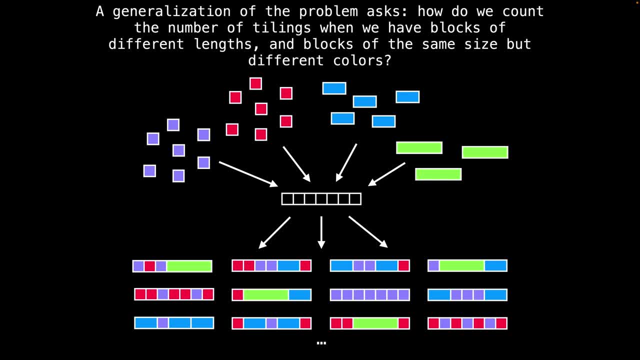 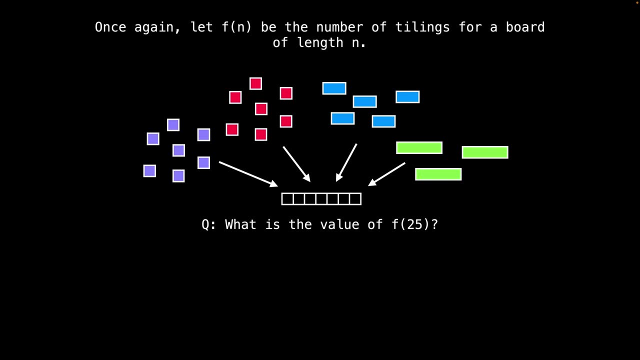 displayed above. You can have a purple block, a red block, a purple block followed by a green block, or maybe two red blocks, two purple blocks, a blue block followed by a red block, and so on. Let's define the function f of n to be the number of tilings for a board. 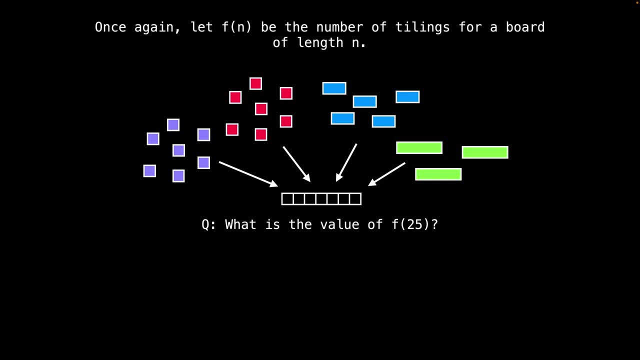 of length n. My question for you is: what is the value of f of 25?? That is, how many ways are there to tile a board of length 25? With the tiles displayed on this screen? I'll give you a moment to think about it, But here are a few hints to get you started. 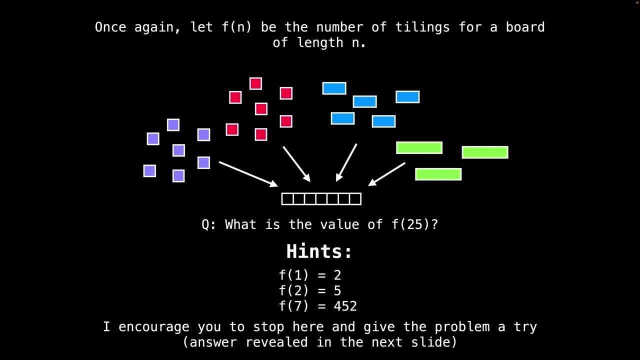 f of one equals two, f of two equals five and f of seven equals 452.. I encourage you to pause the video here and give the problem a try. I'm going to reveal the solution in the following slide. So, according to my calculations, f of 25 is a pretty large number, five billion. 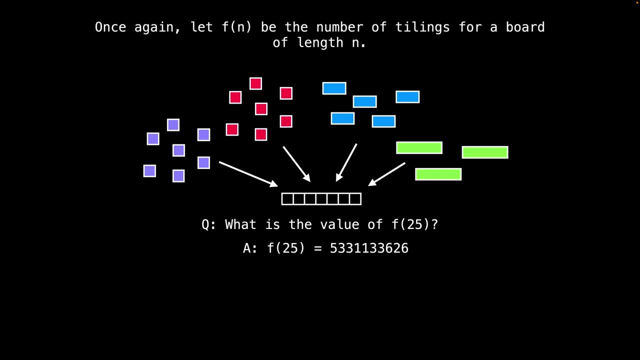 331,133,626.. It's actually not uncommon for these combinatorial dynamic programming problems to yield such large results, because the answers tend to grow very quickly. The approach we're going to use to calculate f of n is to construct all the ways to tile. 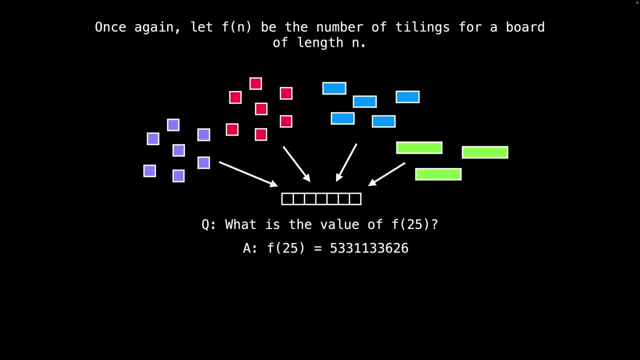 boards of length one, then construct all the ways to make boards of length two, then all boards of length three, and so on. As we do this, you'll notice that we will be able to reuse smaller known board tiling solutions to construct larger boards. We're going to look at how to solve the problem. 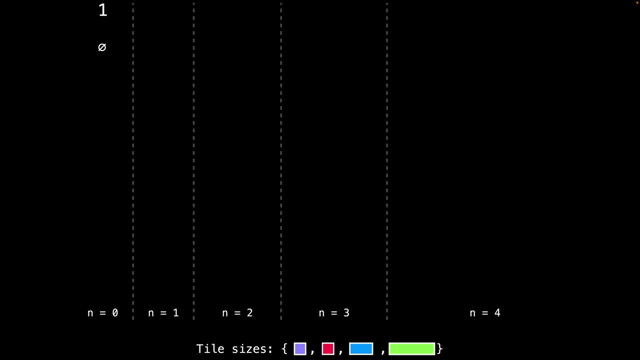 using the bottom up approach we looked at in the last video. First, we need to consider all the ways there are to tile a board of length zero. That may sound trivial, but it's the base case or the foundation by which our dynamic programming solution is based off. 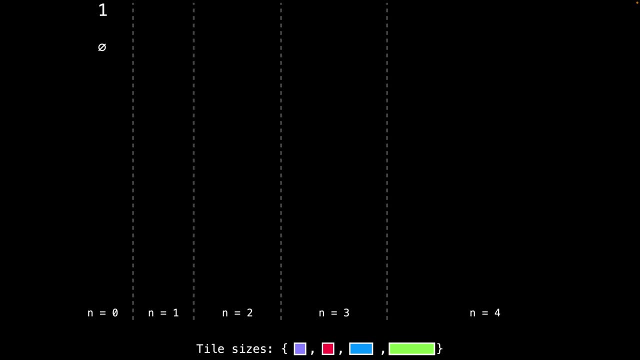 of. So there's exactly one way to make a board of length zero, And that's to have the empty board state From the empty state. there are exactly two ways to make a board of length one. we can either tile the board of length one using a red block or tile a board of length. 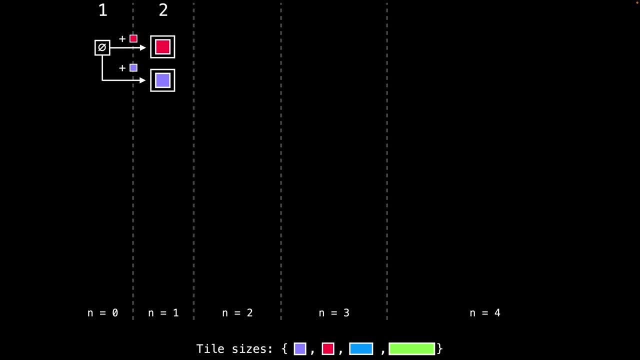 one Using a purple block. there are no other ways to make a board of length one, because our other tiles- the blue and green tiles- are too large to even fit on the board. So we can't even fit on the board at the moment. Next, we're going to construct all the boards. 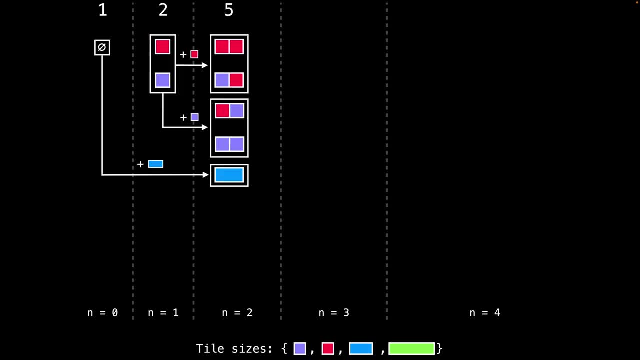 of length two. To do this, we are going to reuse all the solutions from boards of length one to construct boards of length two. by appending a red block to all the solutions, as well as a purple block, you will notice that we are able to create a board with a. 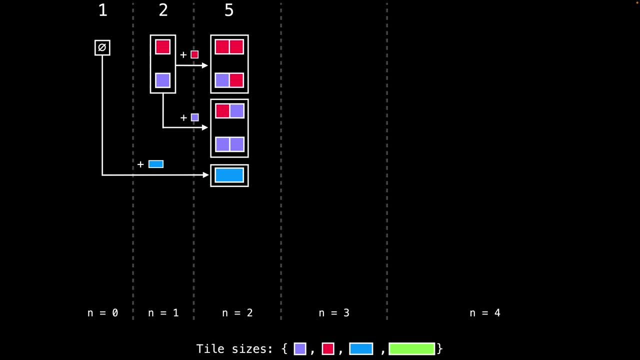 blue tile for the first time. One way to think about this is that we are adding a blue tile to the empty state to create a board of length two. Now you can see that there are exactly five ways to create a board of length two. Next, we are going to construct all boards of length three, Similar to before. 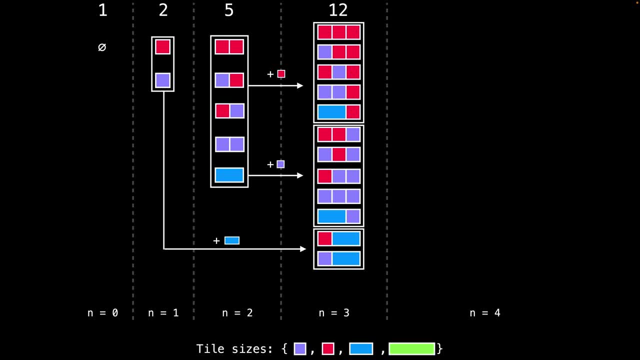 we're going to use all the board tile wings of length two to create boards of length three, By adding a red and purple tile. We're also going to reuse all the board tiles of length two. The next thing is going to use all boards of length one plus a blue tile to create a board of length three. you may. 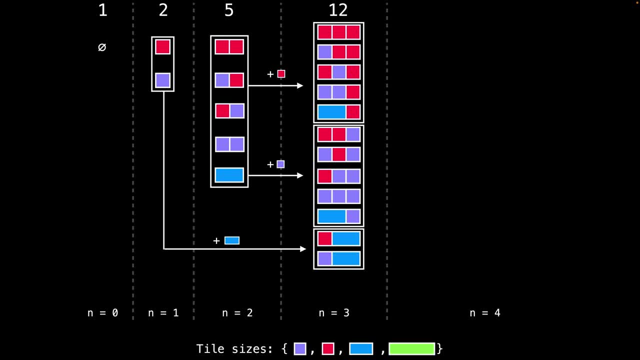 already be seeing pattern here. But essentially for every block of length k that fits on the board we are going to add on all the solutions from k columns ago and add them to the current tiling count. So in this situation there is five plus five plus two for a total of 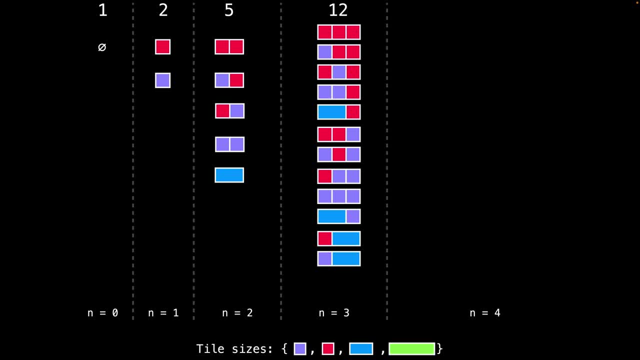 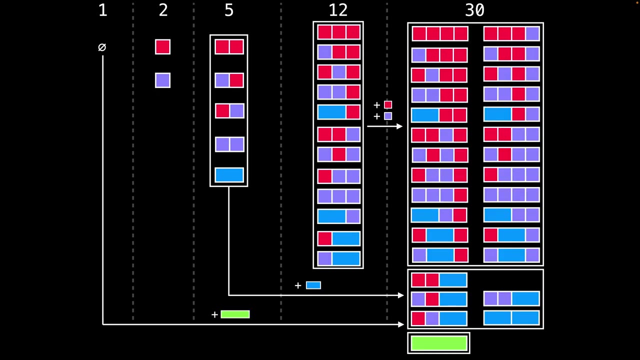 12 pilings of length, three based on the previous example, trying to determine how many ways there are to tile a board of length of four. pause the video if you need more time In order to find all the tilting's for a board of length for a pen. blocks to the existing. 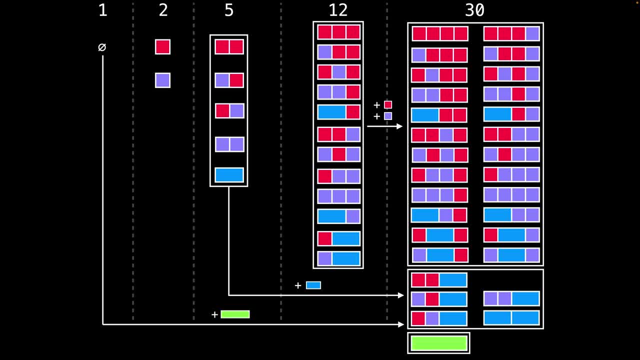 solutions from previous board sizes which result in a board of length for. So in total there are 30 ways to tile a board of length üç, four. Let's take a look at how we might discover the recurrence relation to count the number. 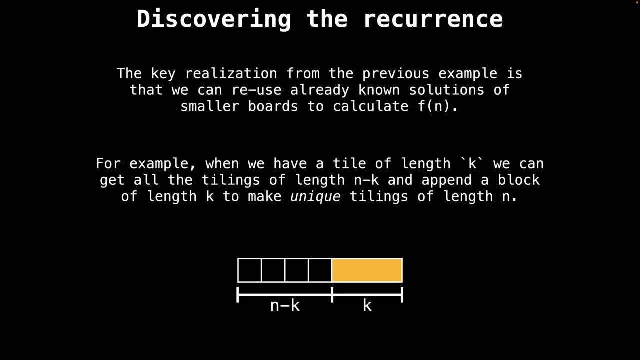 of board tilings. The realization from the previous example is that we can reuse already known solutions from smaller board sizes to compute f of n, For instance, suppose we have a tile of length k that we can use to fill boards. If we get all the tilings of length, 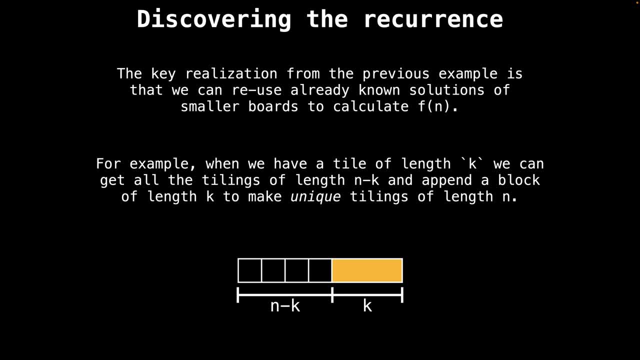 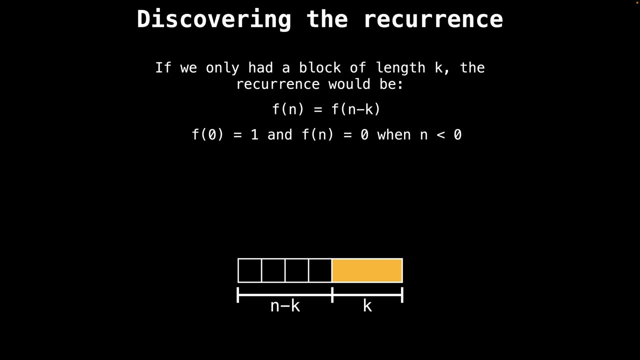 n minus k and append a block of length k, then we have just generated a new unique set of tilings of length n using the block of size k. If you assume that we only had a single block of length k to tile boards with, then the recurrence would be pretty simple it. 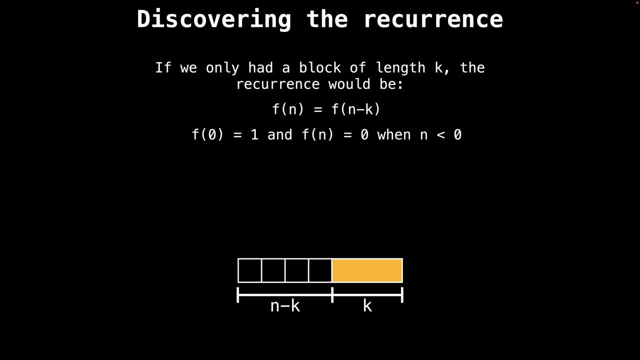 would be f of n equals f of n minus k. However, if we add added another block of length h to our set of available blocks, then the recurrence would become f of n equals f of n minus k, plus f of n minus h, Because blocks of length h are: 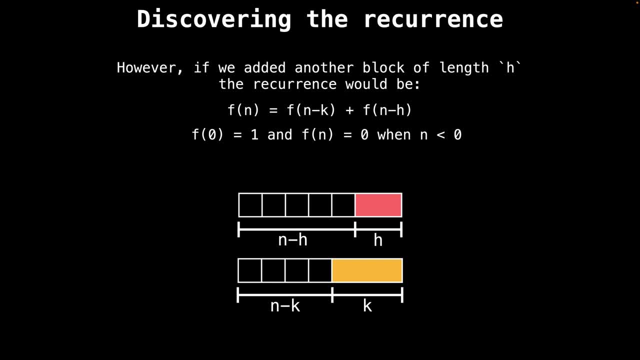 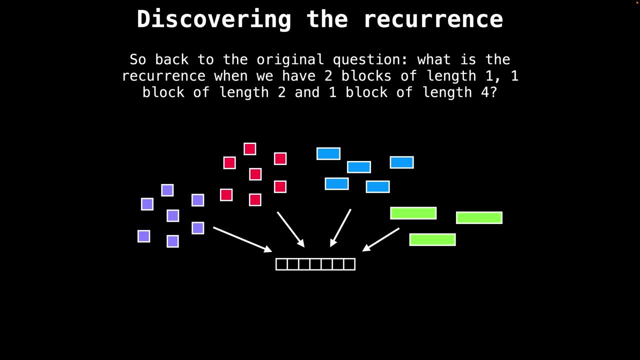 a different color, they generate their own unique set of tilings that need to be accounted for in the recurrence. Coming back to our original question, what is the recurrence when we have two blocks of length, one, one block of length, two and one block of length? 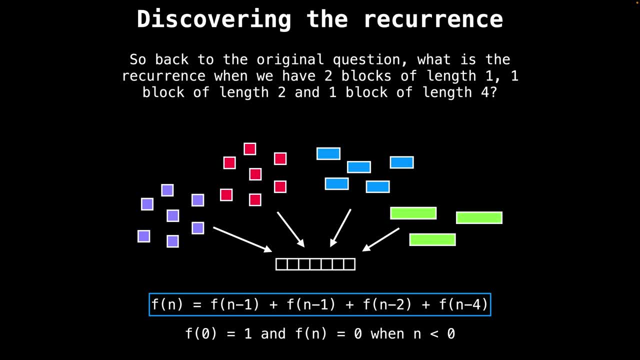 four. Well, in this case the recurrence is f of n equals f of n minus one for the red block, plus f of n minus one for the purple block, plus f of n minus two for the blue block, plus f of n minus four for the green block. Since f of n minus one is repeated, we can: 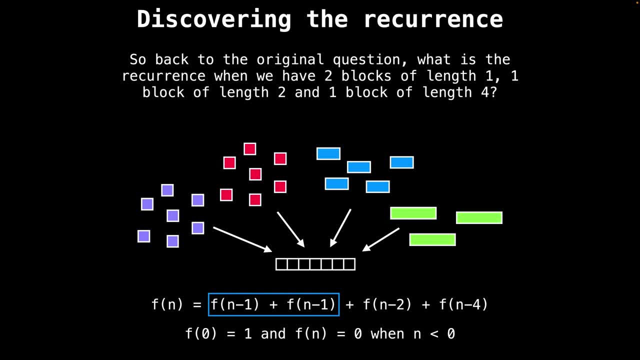 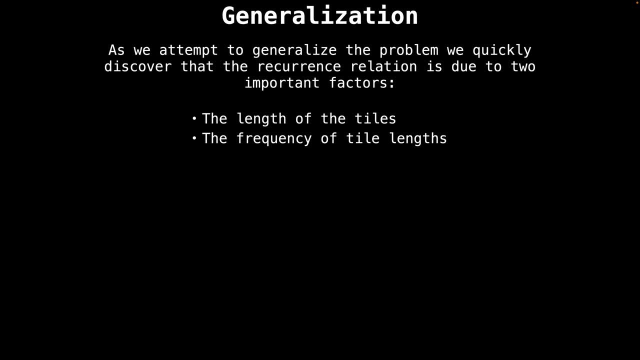 further simplify the recurrence by combining the f of f of n minus one and f of n minus two And minus one terms. This brings us to the generalization of the problem, And as we attempt to derive a general solution, we quickly discover that the recurrence relation is due to two. 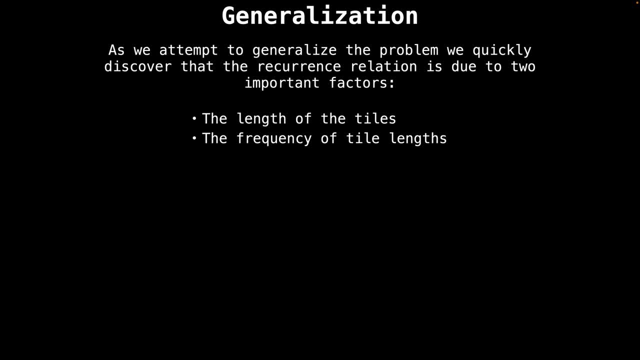 important factors: First, the length of the tiles at our disposal And, secondly, the frequency of the tile lengths. Using that information, we are able to conjure up a linear recurrence which incorporates the lengths of the tiles and the frequency of the tile lengths. The 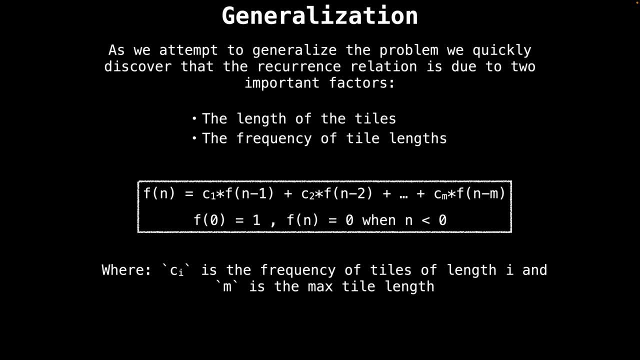 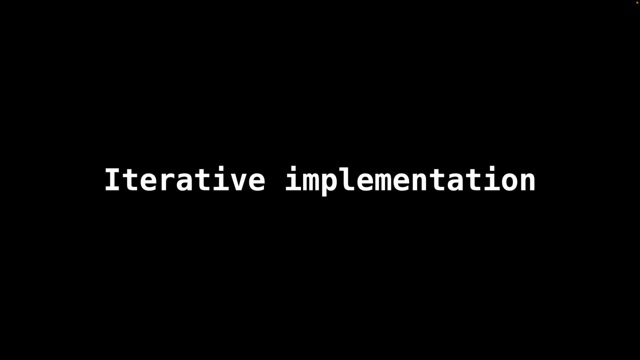 length of the tiles is used to determine the offset in the function to get the board length And the frequency of the tile lengths is used to determine the coefficients in front of the terms in the linear recurrence. Alright, let's take a look at some pseudocode on how to implement the generalized tiling. 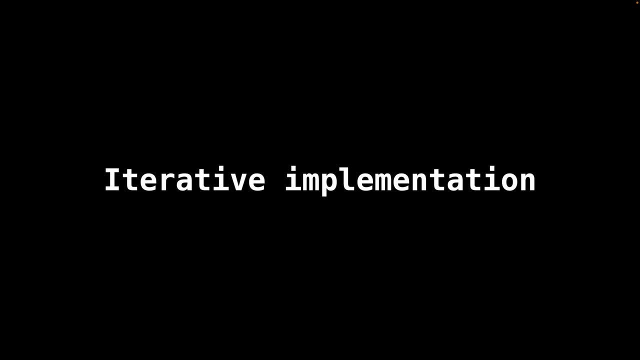 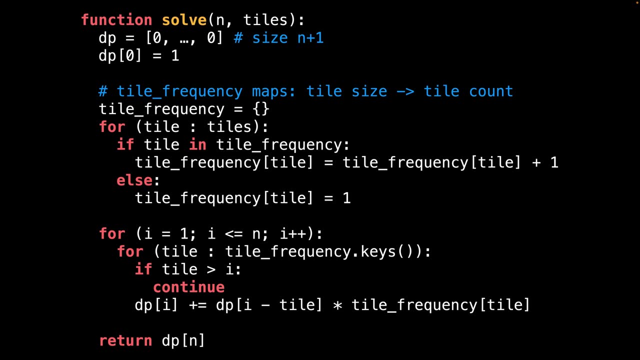 recurrence. Let's begin with iterative solution. This is the code for the iterative solution. The approach here is to use the bottom up solution presented earlier. Let's walk through it As input we provide and the board length we want to solve for, as well as the list containing. 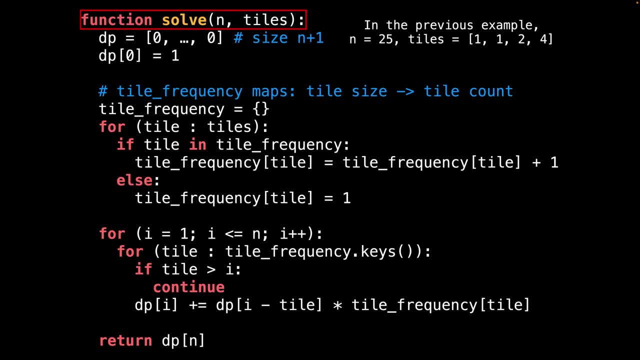 the tile lengths of all the tiles we have at our disposal. In the example at the beginning of the video, we would have specified n equals 25.. And the tiles list equal to the numbers one, one, two and four. To start with, I declare: 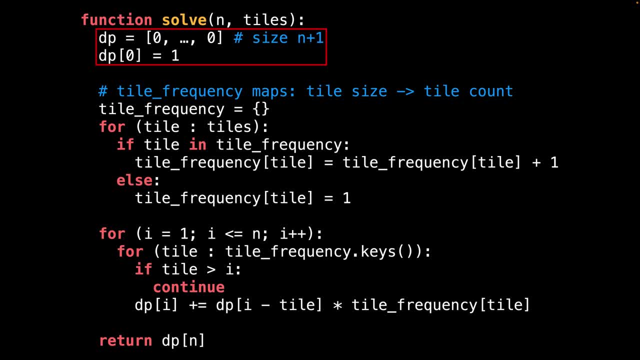 an array called DP, of length, and plus one to store all the solutions, the values of f of n. Since we know the value for f of zero, we immediately set the value of f of zero to equal one as the base case. The next thing I do is declare a map data structure called 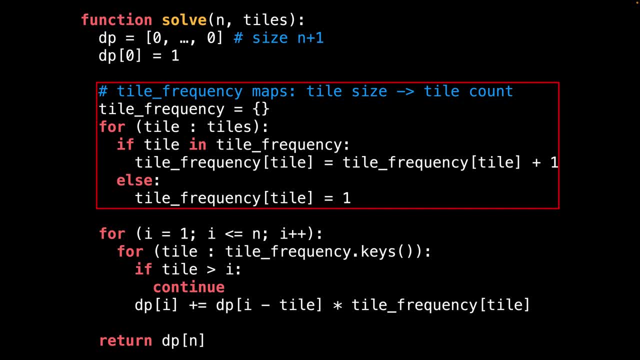 tile frequency, which counts the frequency of each tile length. Then I iterate over all the tiles and count the frequency of each tile length. In this loop the variable I represents the board length. So we iterate from i equals one, meaning border of size one, up to a border of size n. then inside the 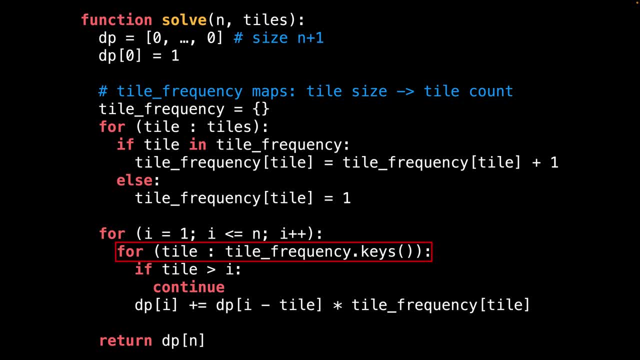 loop. we loop through all the unique tile length, Then we skip the tiles which are larger than the current board size. but to estimate the length of every tile that mayு size, since they can't fit on the board, And sum up the number of ways to tile the board, 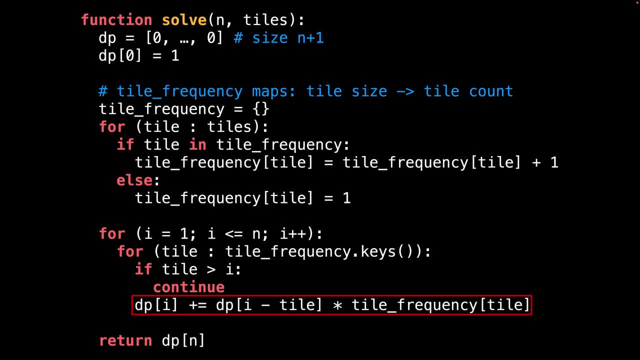 by adding up all the values in the linear recurrence. To do this, we need to add up the number of ways to tile the board at the current length minus the tile size, and multiplied by the frequency of the tile length After the loops have completed the DP array. 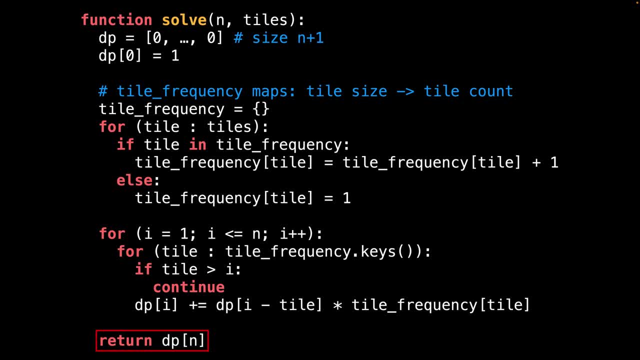 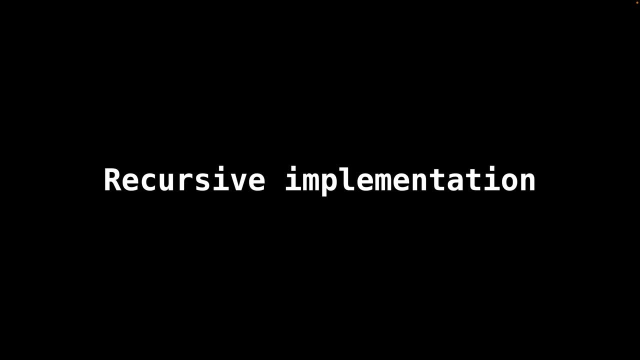 should be populated and we can return the value of f of n. Let's also have a look at the recursive implementation. I think it's important to understand how to implement a problem in more than one way, to expand how you approach certain problems. 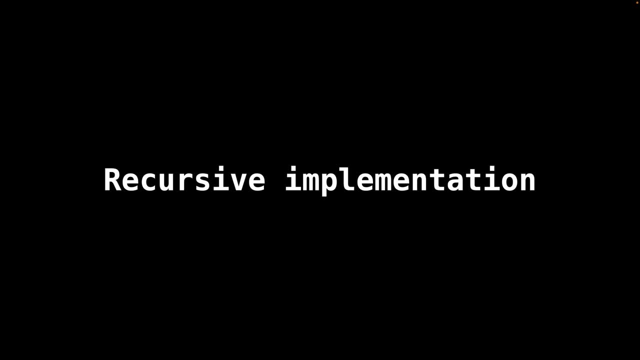 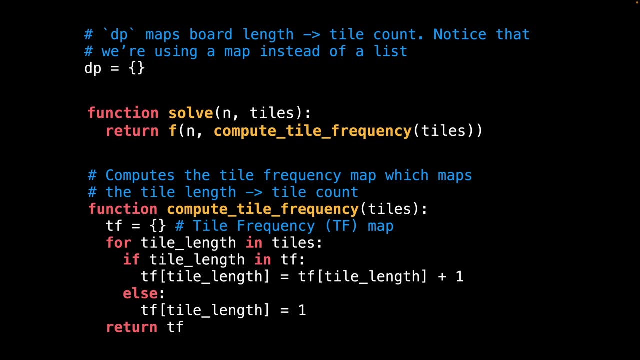 Sometimes a problem will be easier for you if you think about it iteratively. Sometimes it'll be easier for you if you think about it recursively. The idea behind the recursive implementation is largely the same concept, except that, instead of solving the problem bottom up, 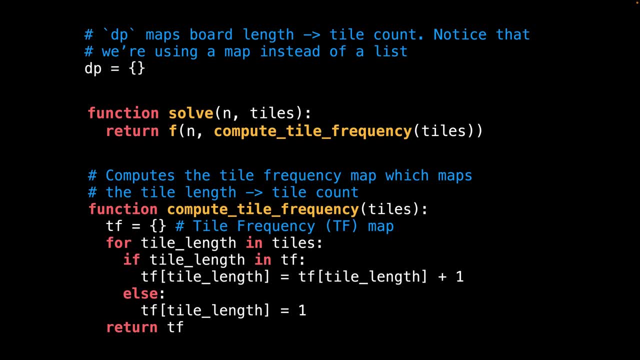 we're going to be solving it top down. To do that, we are going to break the board down into smaller boards instead of building larger boards from smaller boards. On the first line, I declare a map called DP, which maps the board length to the tile count. 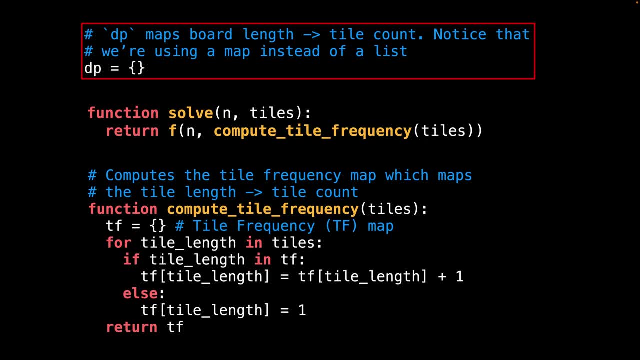 This is where we will be storing our solutions. I decided to use a map instead of an array because it's possible that the number of subproblems is very small. This can happen when the tile size is quite large, And by using a map, we can save some memory. 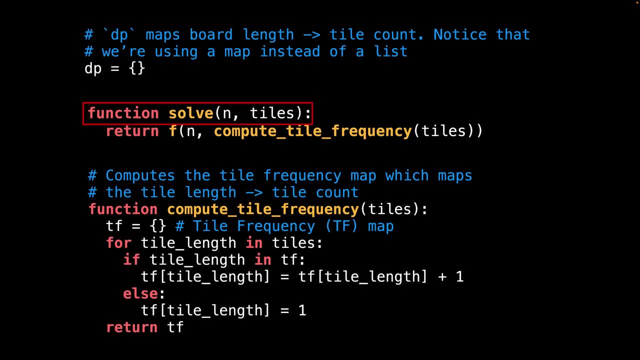 when the value of n is very big. The recursive implementation takes the same inputs as the iterative approach and the board size, which is 1, is very small, So I can set the size And of course the size is very small. 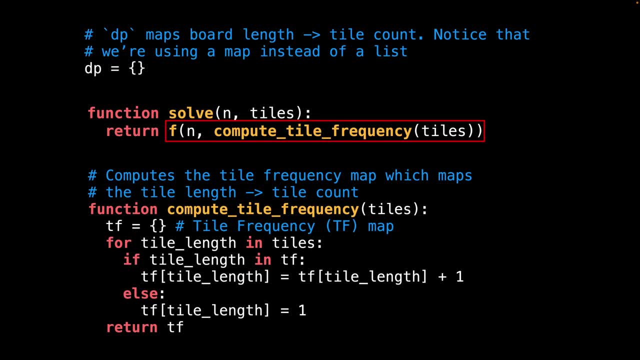 so we will set the size, But for now we will work on the unit size and the tiles array Inside the solve function. all I do is stage a call to the recursive function f. In addition to the board length, I also provide the tile frequency. 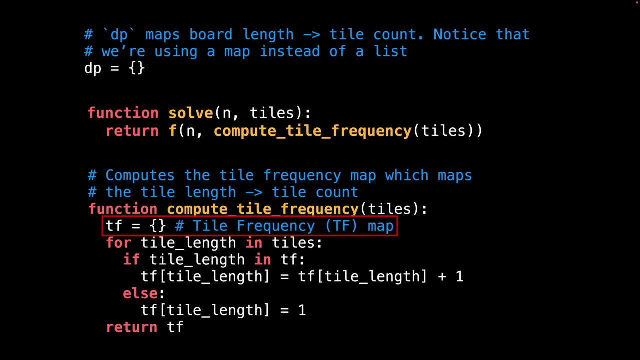 map as another argument to the function Which gets calculated below in the compute. First we declare a map called tf, short for tile frequency, which maps the tile length to the number of tiles of that length. Then we do a simple loop through the tiles and 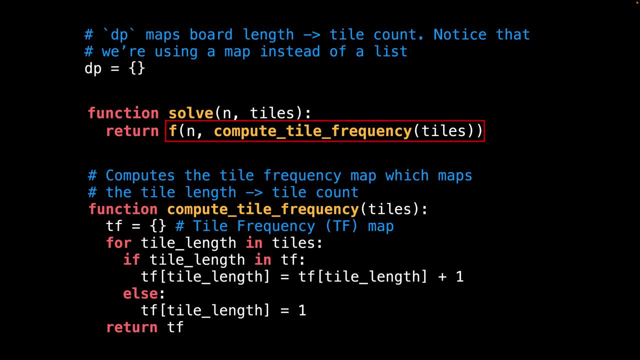 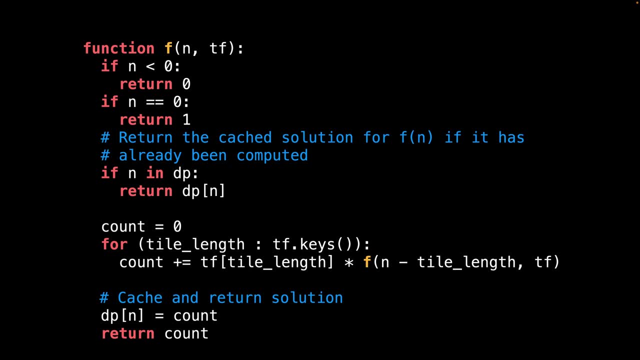 compute the frequency for each tile length. Now let's take a look at the recursive function itself, which is what actually computes the different board tiling configurations As input to the function we provide, and the current board length and tf- the tile frequency. 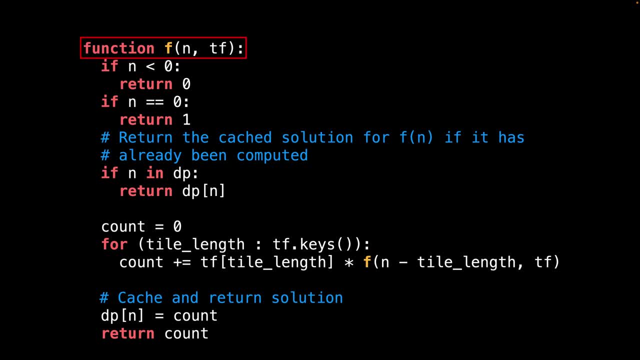 of each tile length. the tile frequency map is actually constant. you could pull it out to simplify this function if you want it to. The first thing I do is check if the board length is constant. If it's not, then I'm going to check if the board length is. 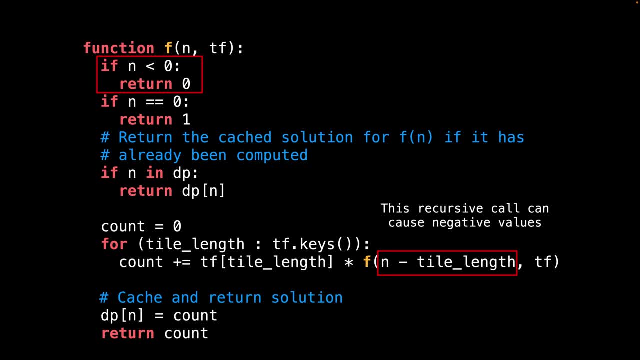 constant. If it's not, then I'm going to check if the board length is constant. If the board length is negative. if so, return zero to indicate that we were able to produce zero board tilings. it is possible to get a negative board length when we subtract the tile length from. 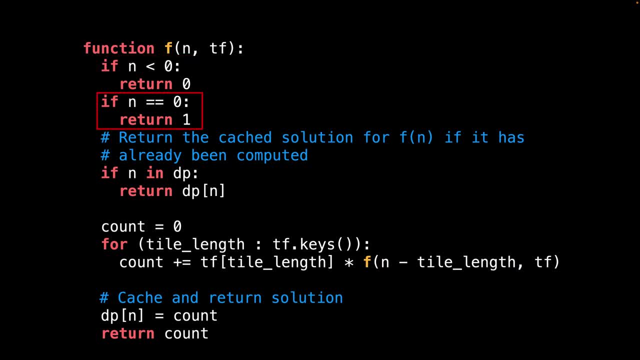 the board size in the recursive call below. Next we check if we have successfully completed tiling a board. If so, we can return that there was exactly one way to tile the board using the tiles that were placed. The next thing we do is check the cache to see if we have already computed the solution for f of n and return a.